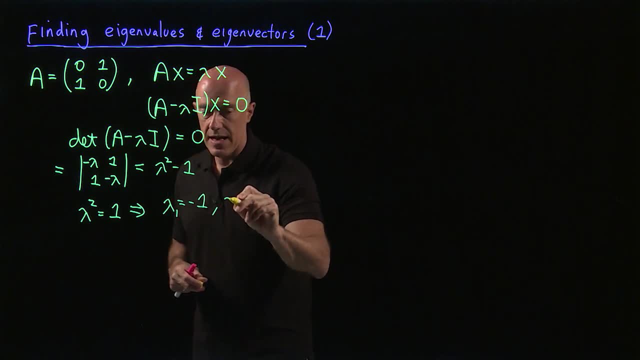 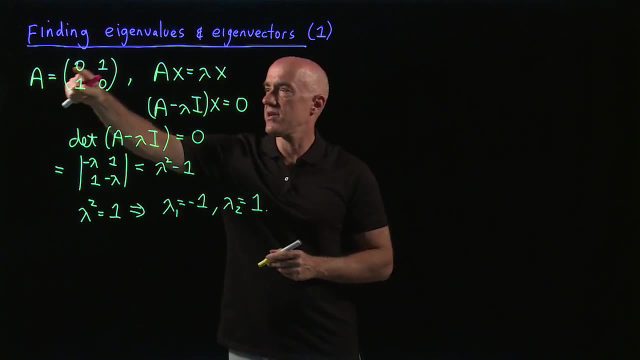 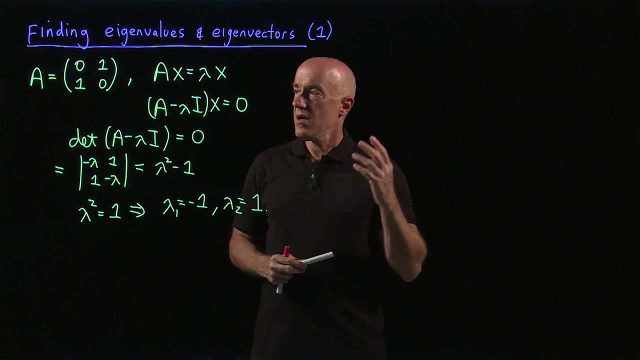 Lambda 1 equal to minus 1, and lambda 2 equal to plus 1.. So this matrix A- 0, 1, 1, 0, has two eigenvalues: minus 1 and plus 1.. We want to find the eigenvectors. 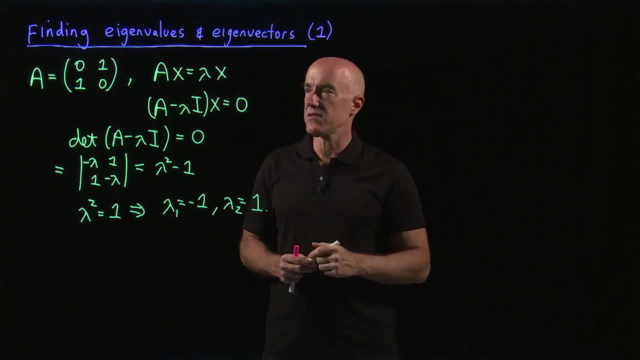 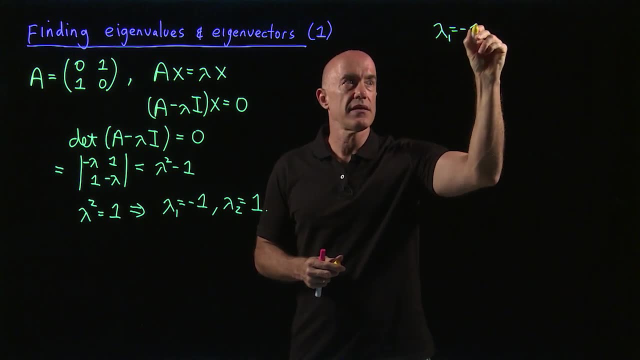 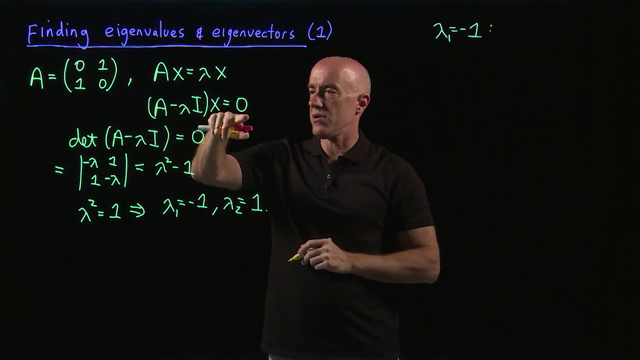 So each eigenvalue has an associated eigenvector. So how do we find the eigenvector? So if we start with lambda 1 equals minus 1, we go back to this A minus lambda i x equals 0.. Now we're looking for lambda i x equals 0.. 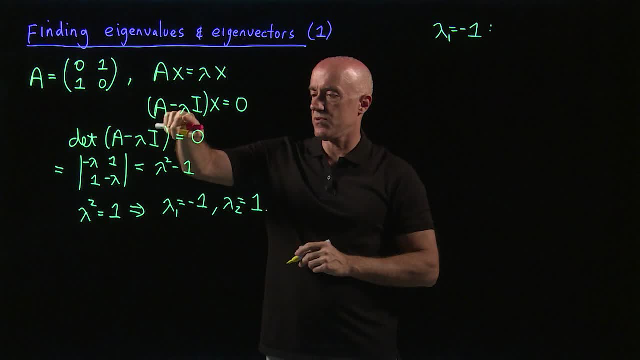 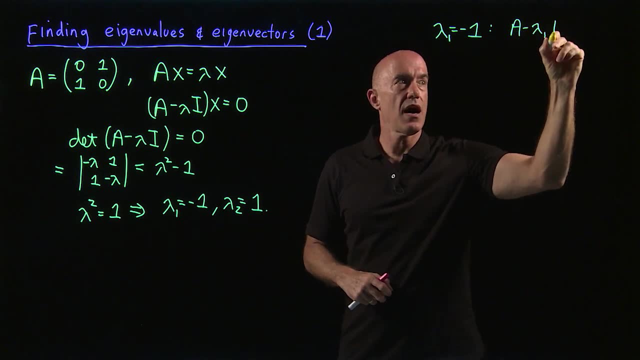 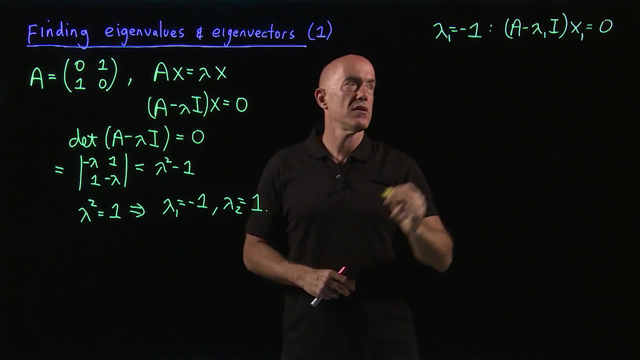 We're looking for the x associated with lambda equal to lambda 1.. So the equation we want to solve is A minus lambda 1, i, And the eigenvector here would be x1 equal to 0.. So this is the equation for the eigenvector. 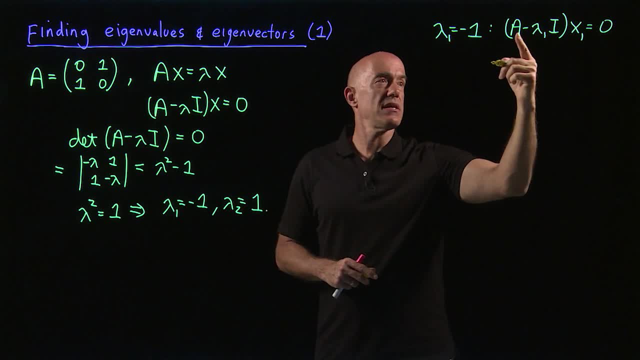 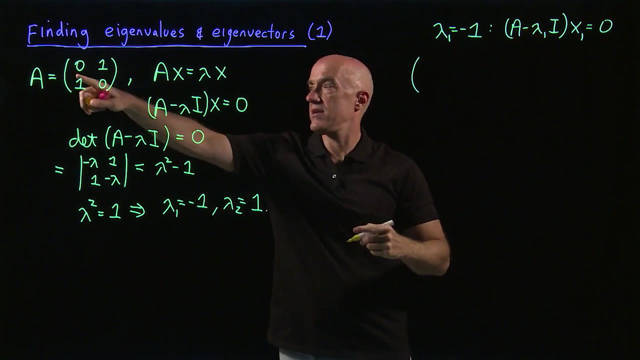 Lambda 1 is equal to minus 1.. So this means A plus i. We add 1 plus 1 to this, So the diagonal elements of A. So this is a matrix equation. I can write that as A plus i. Here's our A. So I'm adding 1 to the diagonal elements. 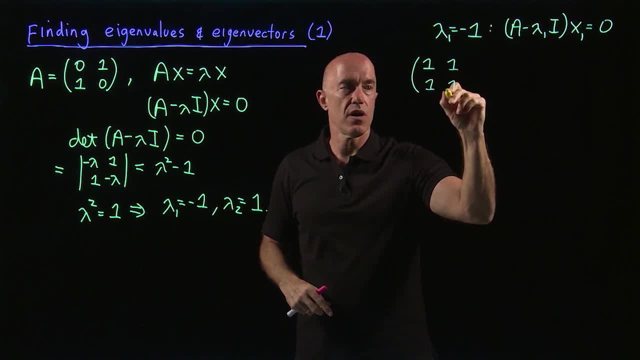 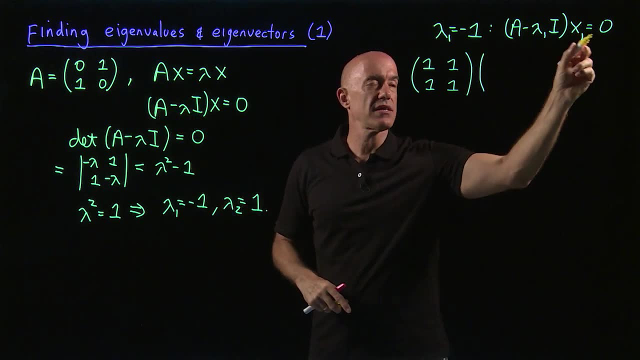 So 1, 1, 1, 1.. That's A plus. i right times x1.. Let me call x1 here. I'm going to call v1, v2.. So these are the components of x1.. 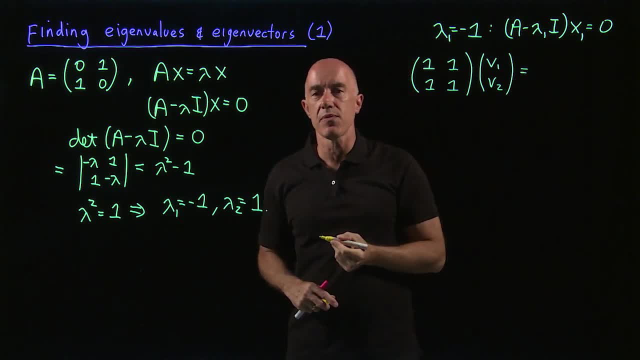 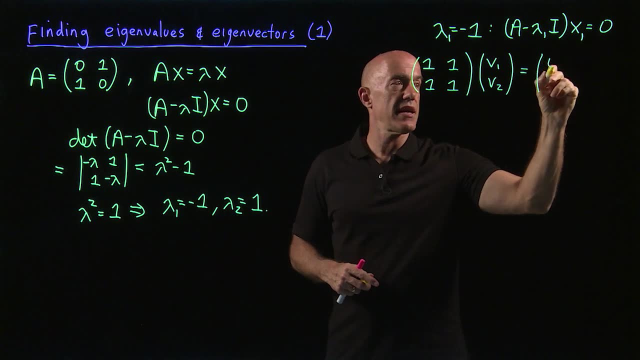 And this is supposed to be 0. So remember, 0 is a special symbol that can be a matrix or a scalar. Here, of course, it's a column vector, right? So that's our 0.. So this is two equations, right. 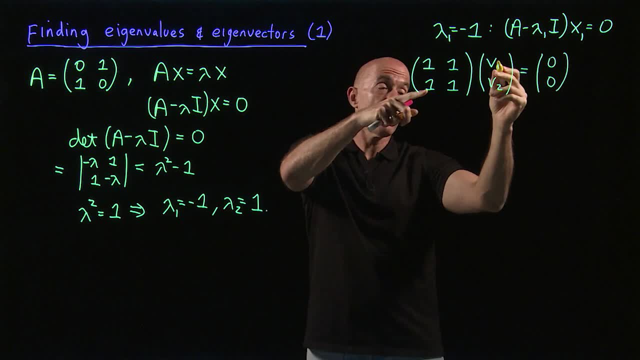 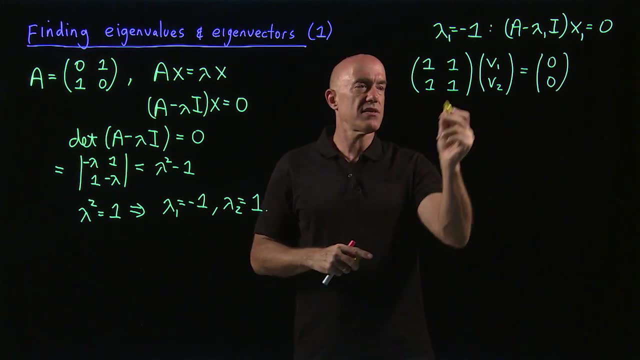 v1 plus v2 equals 0. And v1 plus v2 equals 0. So actually the second equation is exactly the same as the first equation. That's always true. The second equation is always the same. There's always just a multiple of the first equation for the 2 by 2 case, because this: 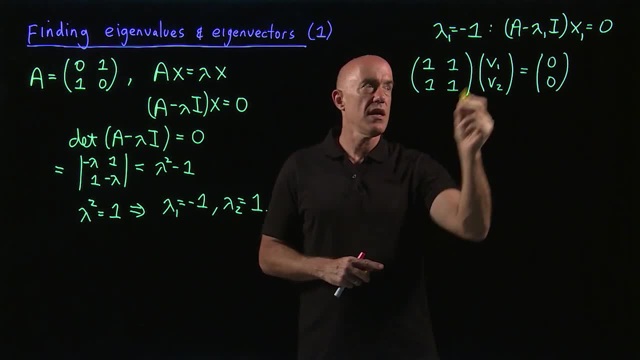 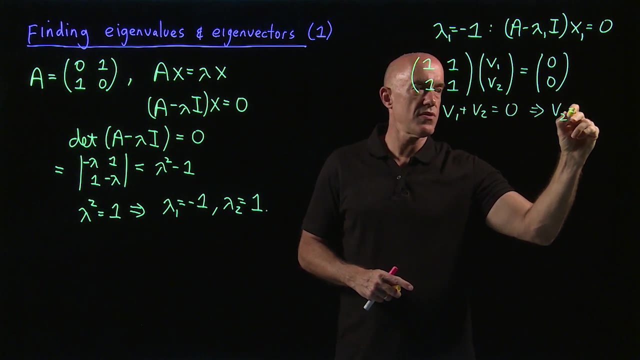 matrix is not an invertible matrix, right? Remember? A minus lambda i is not an invertible matrix. So we get: v1 plus v2 equals 0, which tells us that the second component is equal to the negative of the first component. okay, 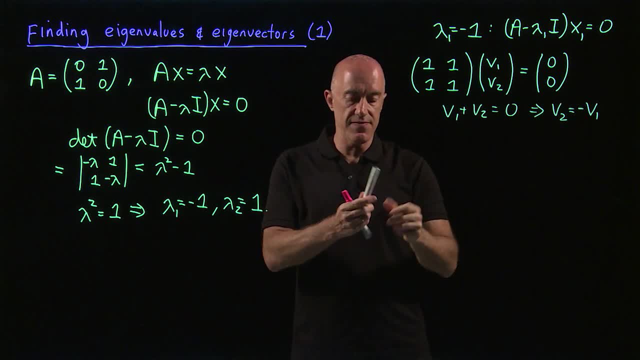 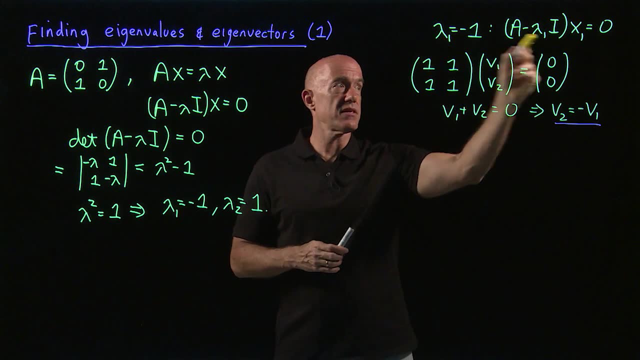 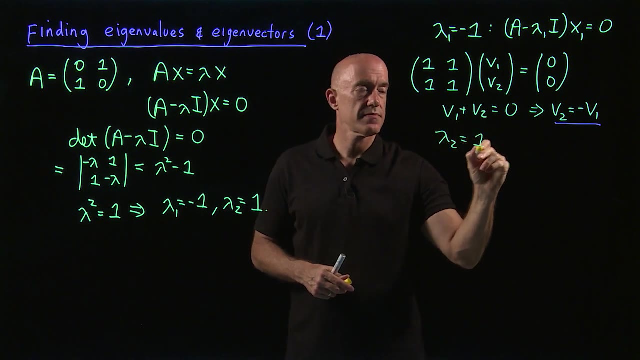 So that's for the eigenvector. So let me just leave this. I'll close that like this and then we'll write down explicitly the eigenvector at the end. Okay, that's the first eigenvalue. The second eigenvalue: lambda 2, equals 1.. 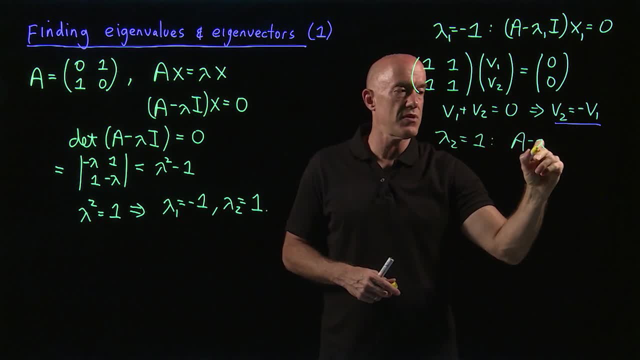 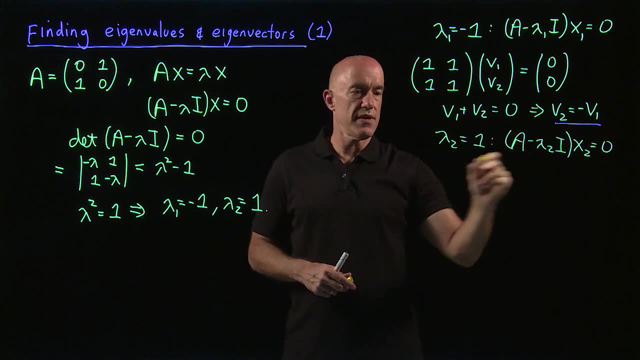 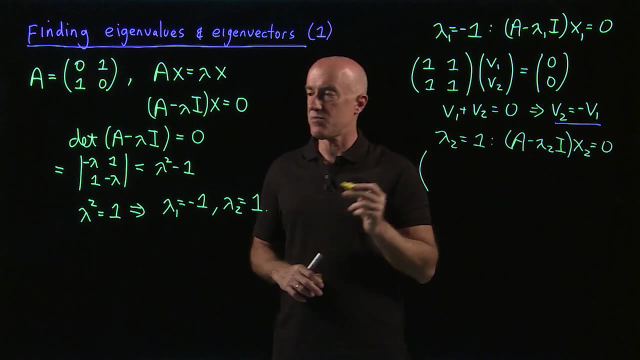 The same equation, right. This time we have A minus lambda 2i times. the second eigenvector is equal to 0. This matrix equation tells us lambda 2 is 1.. So that means A minus i. so we subtract 1 from the diagonal elements of A, So we get. 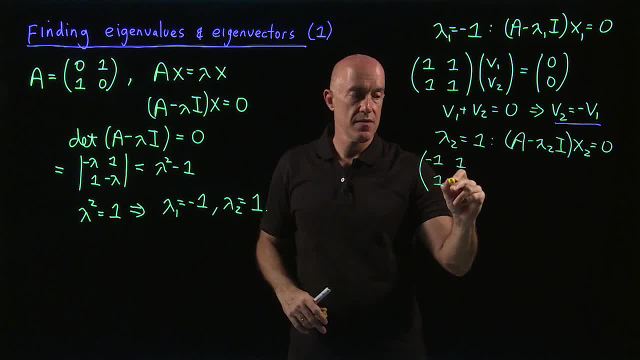 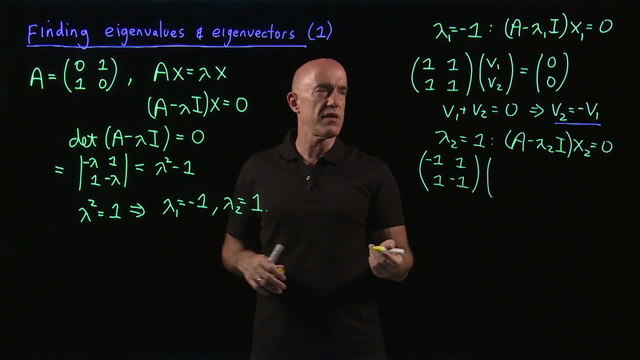 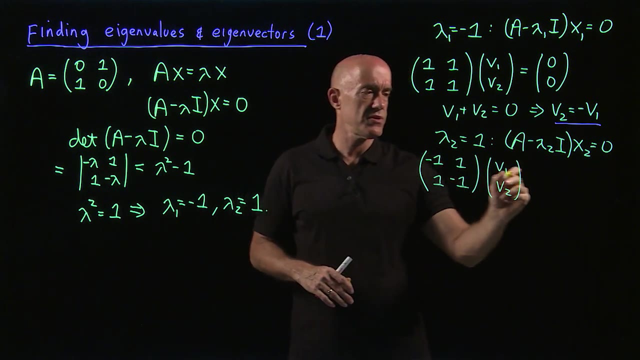 minus 1, 1, 1, minus 1 times the eigenvector. Let me just reuse the symbol v1 and v2, okay, even though they have different values here, But for simplicity I'll just reuse those symbols. and that's supposed to be equal to. 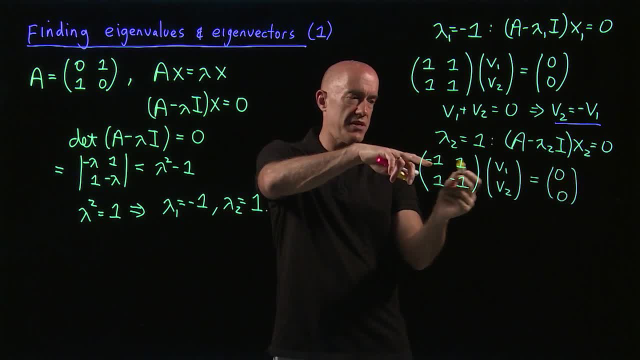 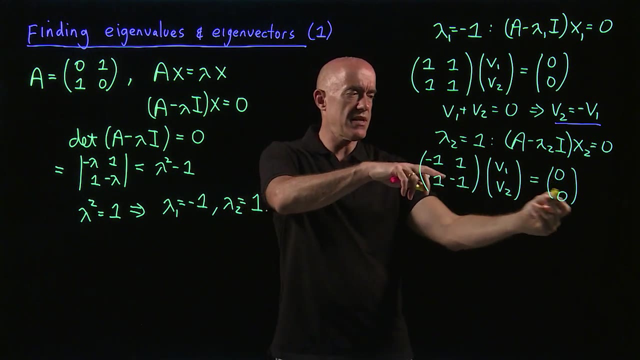 0.. Okay, So here the first equation is minus v1 plus v2 equals 0.. The second equation is: v1 minus v2 equals 0.. The second equation is just the negative of the first equation, So again, doesn't add any additional information. 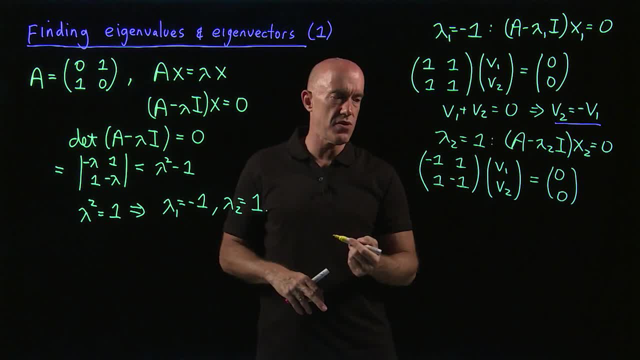 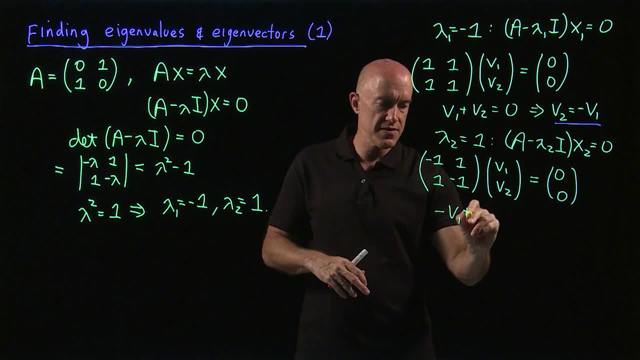 That has to do with the fact that the determinant of this matrix is 0.. So then, what is the first equation? We can start with the first. So minus v1 plus v2 equals 0.. Okay, So v1 plus v2 equals 0. 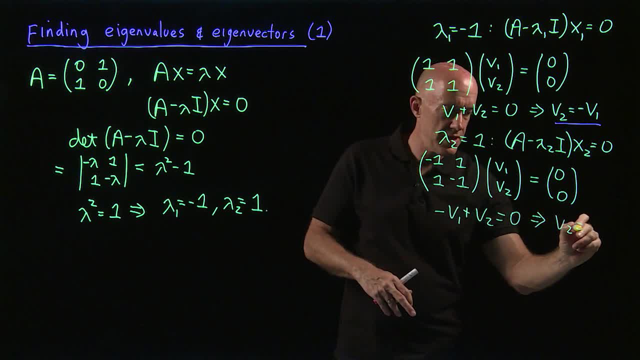 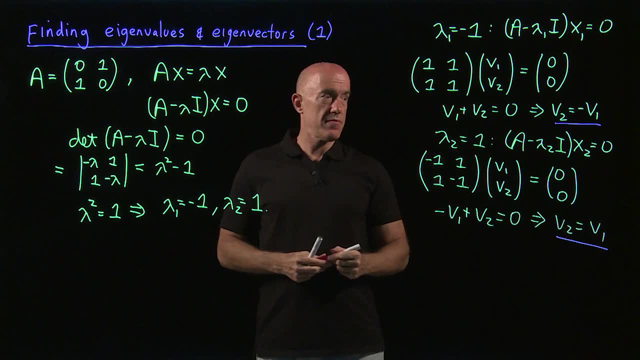 And here we can solve for v2.. So here v2 is equal to v1, okay, All right. So this gives us the eigenvectors and we have the eigenvalues. I can put this together, So let me put it down here. 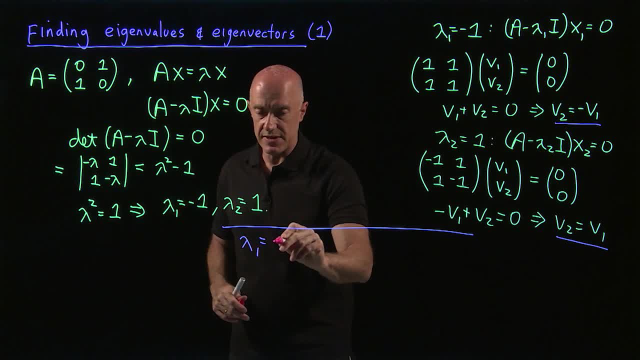 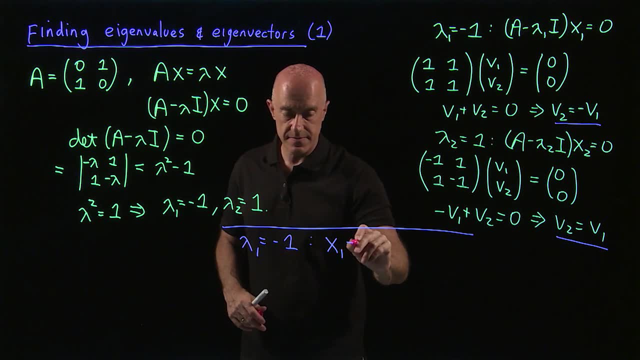 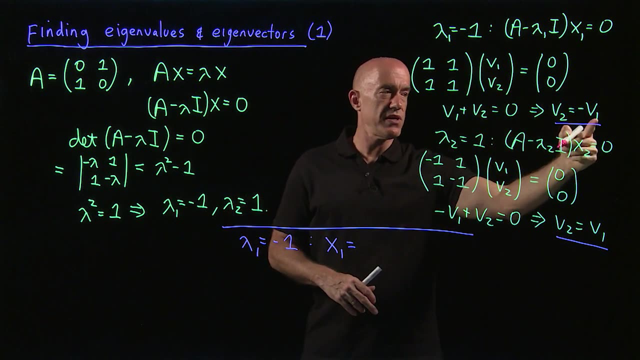 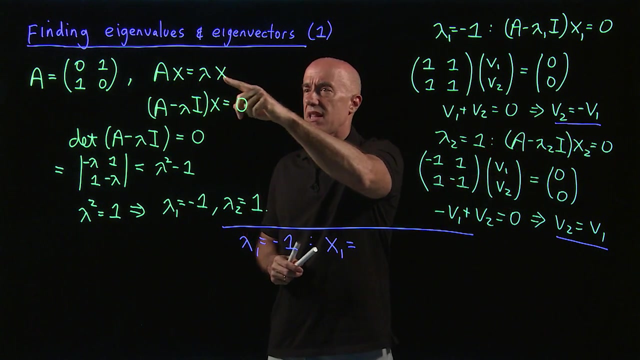 We have for the first eigenvalue, lambda 1 equals negative 1.. And then for the first eigenvector, x1, the eigenvector associated with lambda 1 satisfies: v2 equals minus v1.. So we have a freedom of a constant here, because ax equals lambda x. 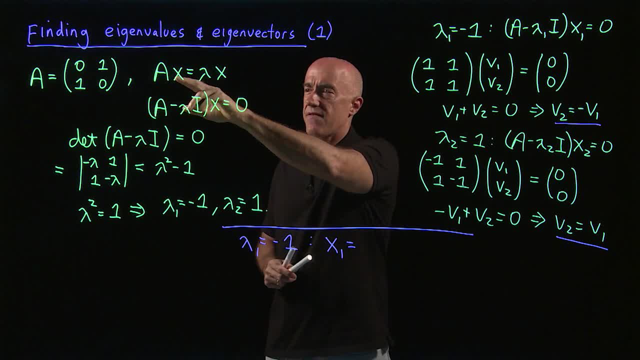 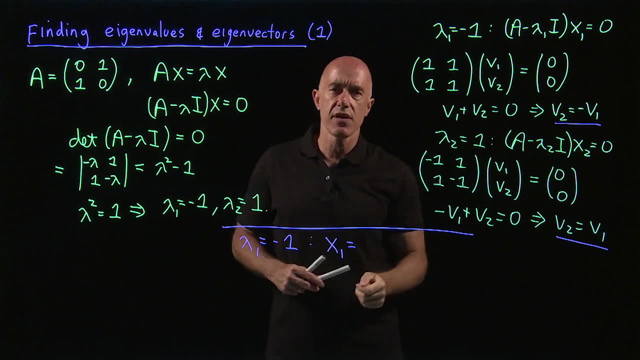 If we multiply x by a constant, we still have a times cx equals lambda times cx- Still the same equation. So the eigenvector is only determined up to a constant. okay, That means we can normalize the eigenvector. Sometimes we're going to want to normalize it. so the norm is 1.. 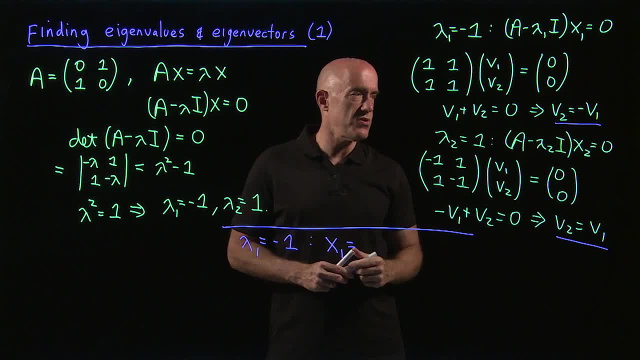 In this case it doesn't matter. So in this case, what I want to do is to set just v1 equal to 1, okay, So that's the simplest thing to do. So v1 is equal to 1.. Then v2 is equal to 1.. 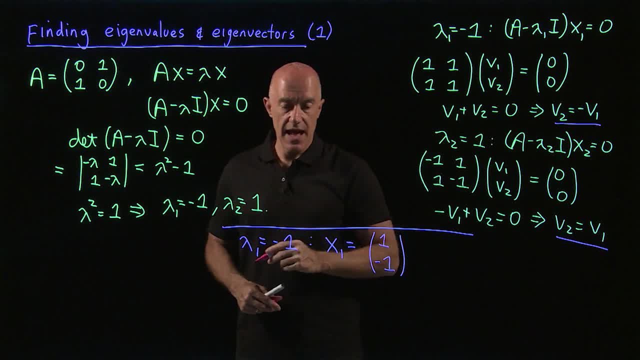 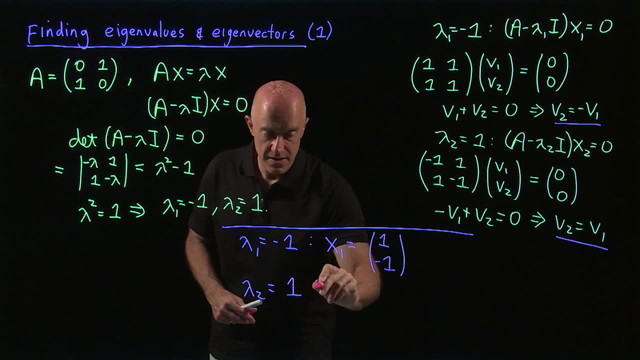 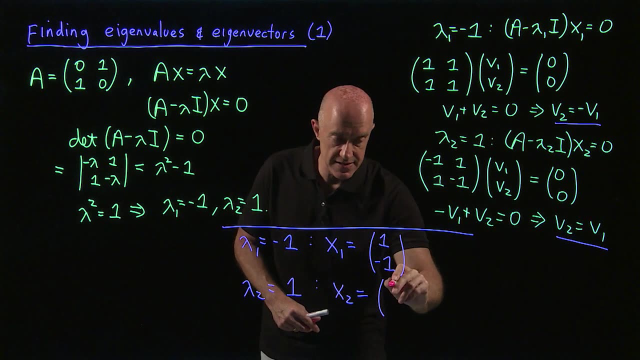 Then v2 is equal to negative 1.. And that's the eigenvector. And then the second eigenvalue, lambda 2 equals plus 1, we got x2. then comes from here v2 is equal to v1.. So here I can set v1 equal to 1.. 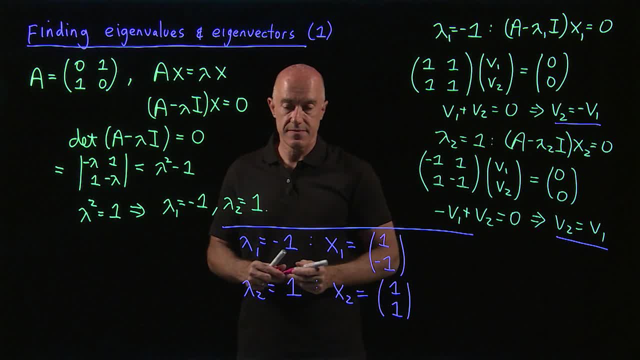 And then v2 is the same, so is also 1.. Okay, You can try this. You can take a. You can multiply by x1. You should get negative 1 times x1. So a times 1 minus 1 should give you minus 1, 1.. 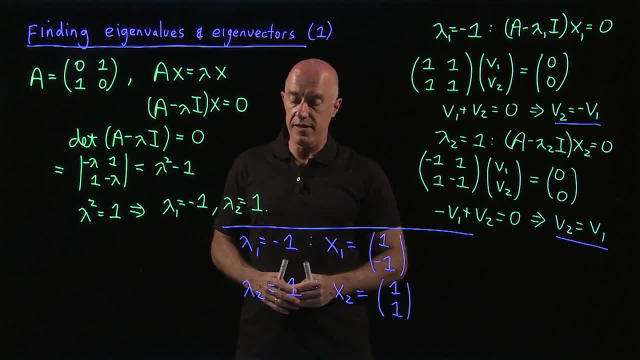 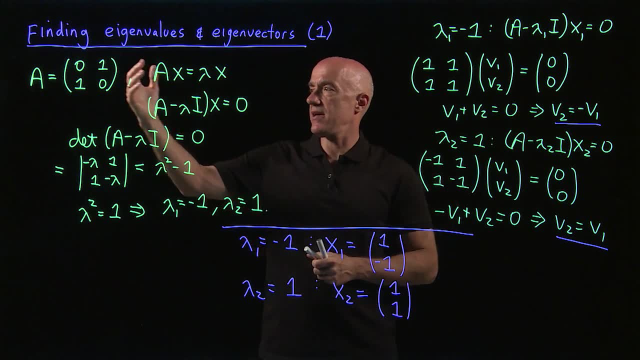 And a times 1, 1 should give you 1, 1, because lambda 2 equals 1.. Okay, So what have we done? We considered a symmetric matrix a 0,, 1,, 1, 0.. 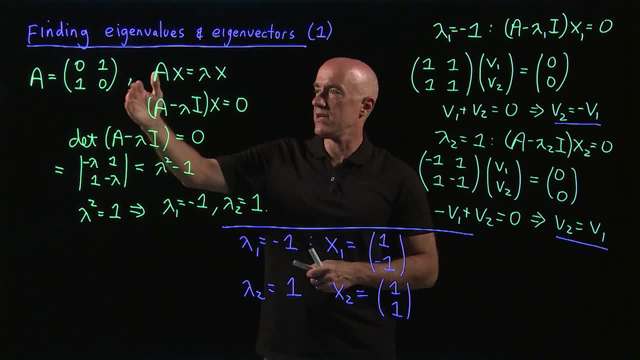 Symmetric matrices can be proven to have only 1.. There is no real eigenvalues. So we work the eigenvalue problem. ax equals lambda x. We find the eigenvalues. There are two eigenvalues minus 1 and 1..